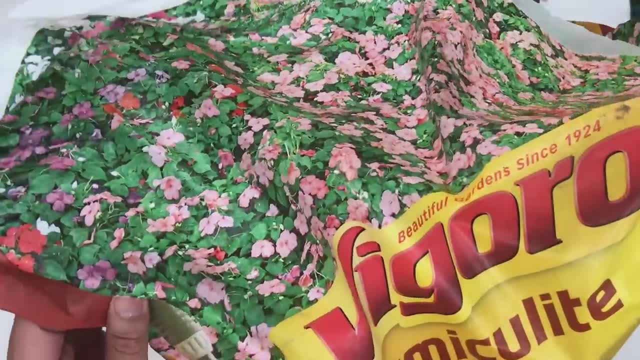 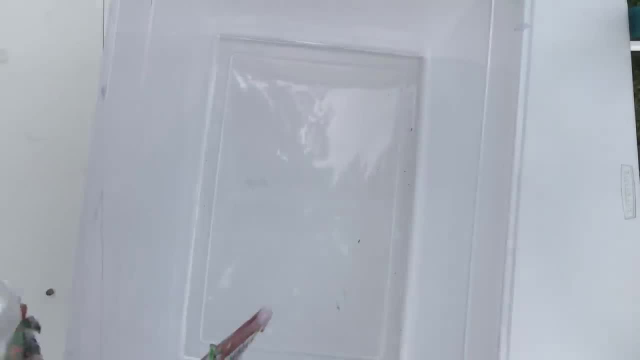 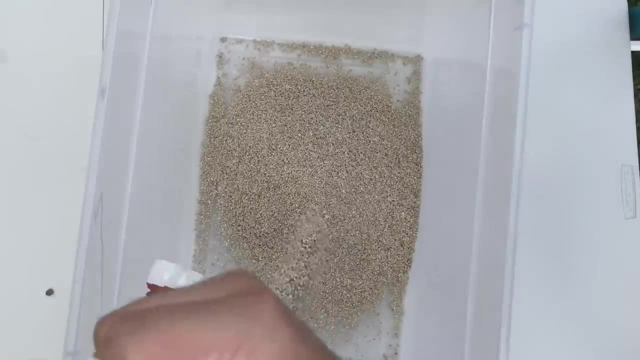 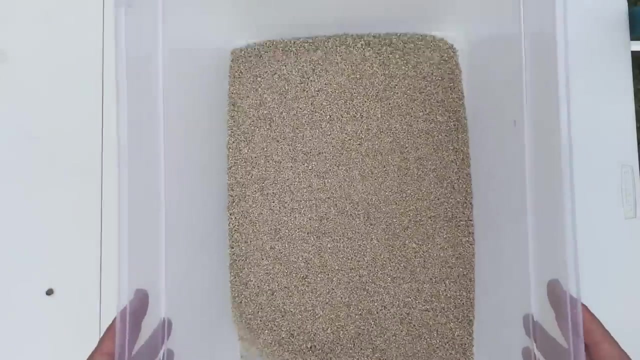 stuff is very light And practically no weight to it at all, So what you're going to want to do, then, is take your tub and line maybe about the first two inches with the vermiculite, just so you have a nice substrate for your crickets to move around on. There we go, Spread it around. 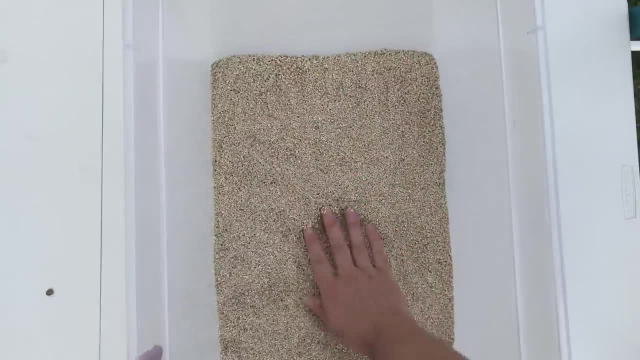 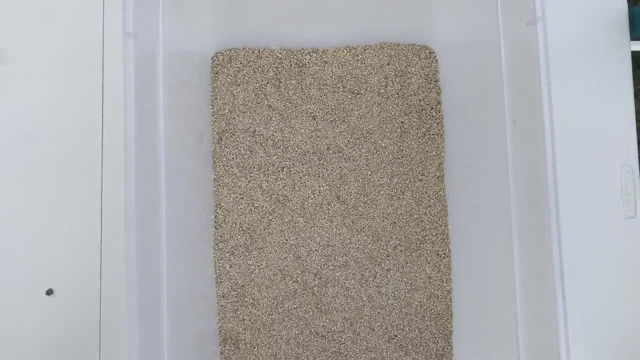 There we go, There, we go, There we go. So so, looking aside, yeah, it might be an inch, Probably, go a little heavier. Crickets aren't going to burrow in it, They just use it to walk around on. And the benefit of using 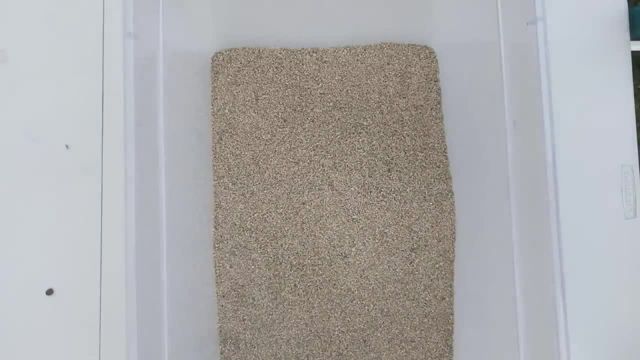 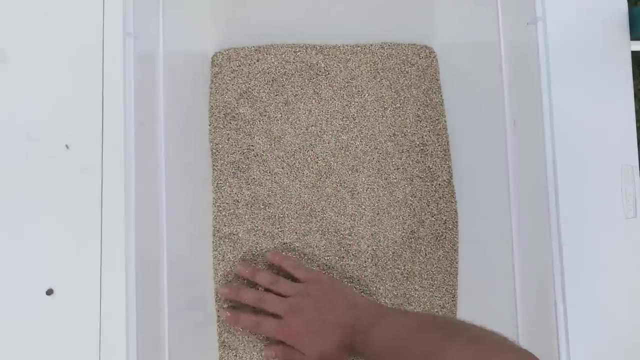 this is that it's very absorbent. So when the crickets defecate and go to the bathroom, this is going to control that odor. So that's, this is perfect. This is what you want: Large plastic tub with a small tub. 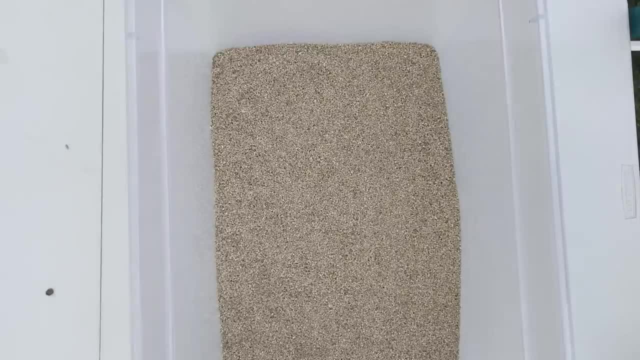 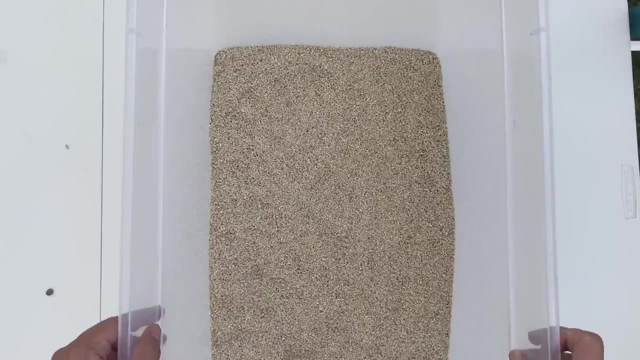 With some vermiculite on the bottom. So this is step number one. The next step is when you raise your crickets, they need a separate substrate to lay their eggs in, And that other substrate is topsoil- Topsoil. 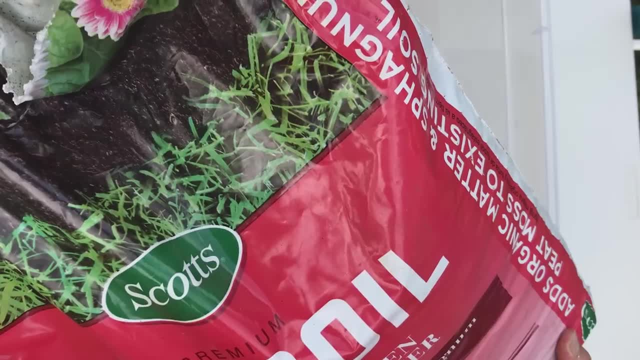 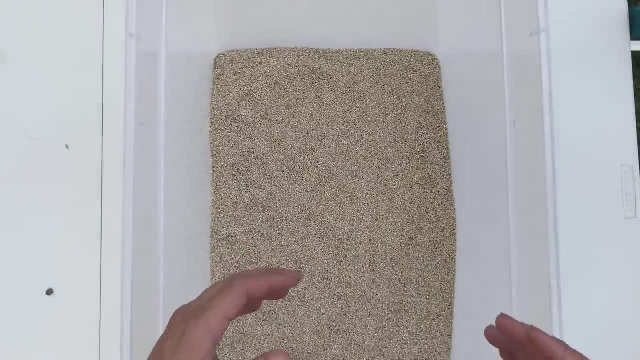 is a lot denser. It's a lot denser than vermiculite. It retains moisture a lot better With these cricket eggs. You're going to need those cricket eggs to be in a nice humid environment And that that topsoil is going to help keep the humidity up. 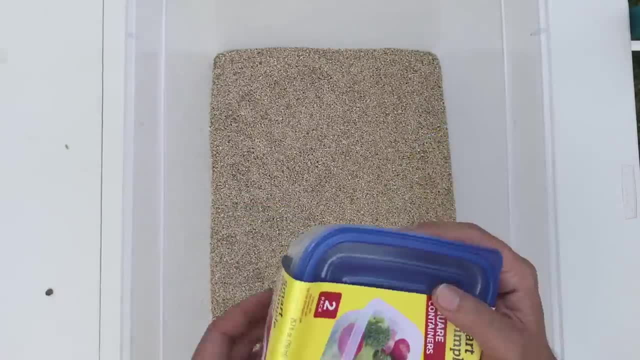 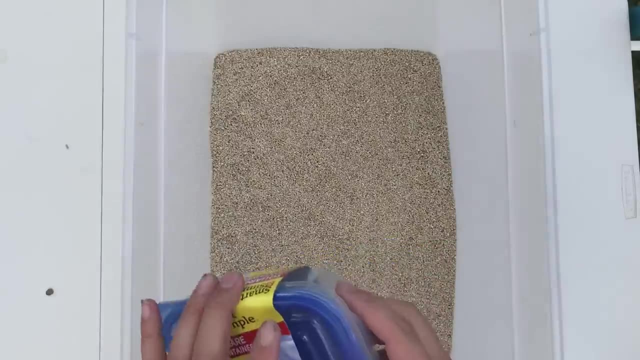 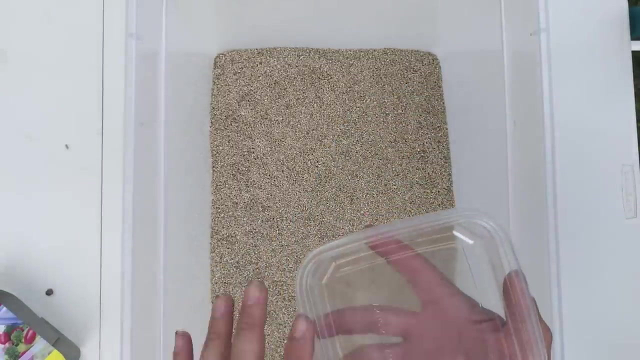 So you know something: you can use Tupperware. I got this Tupperware at the dollar store and this is a perfect size. This is just a sandwich Tupperware package, So what you want to do is just just take one of them like this: You want to fill it with your topsoil. 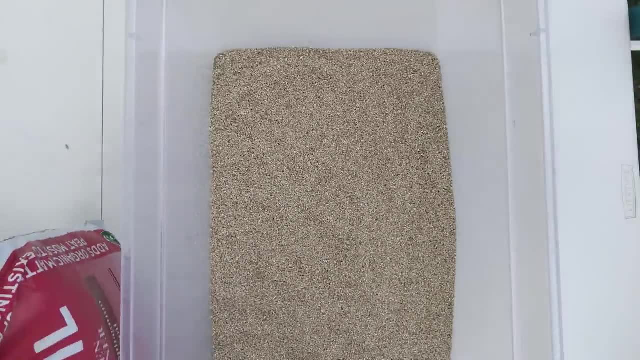 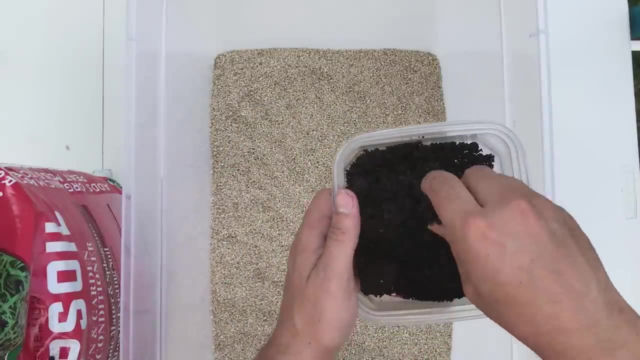 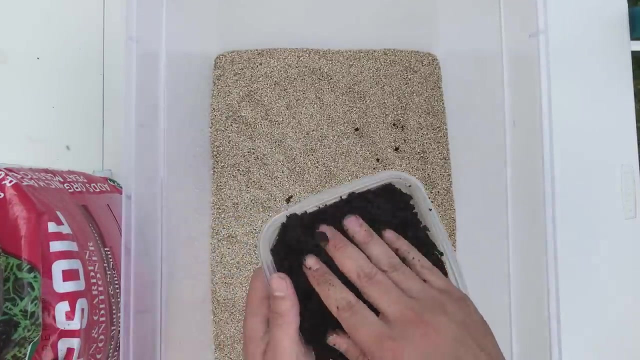 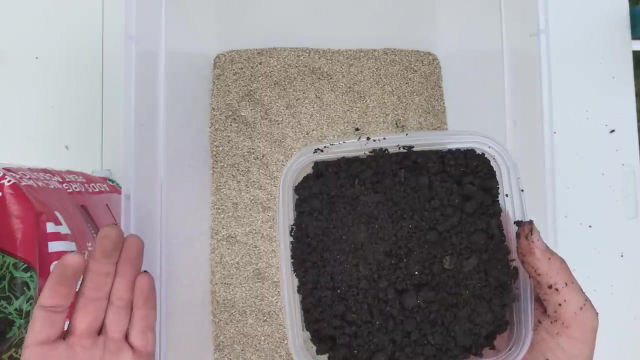 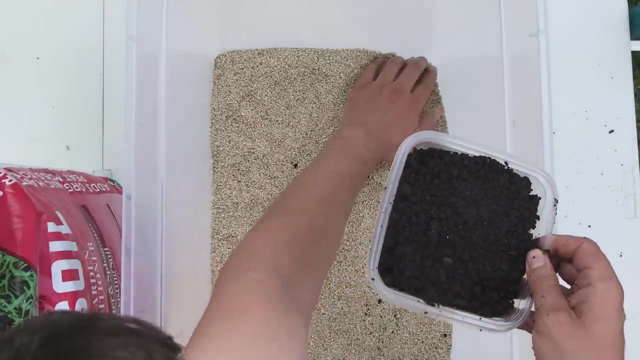 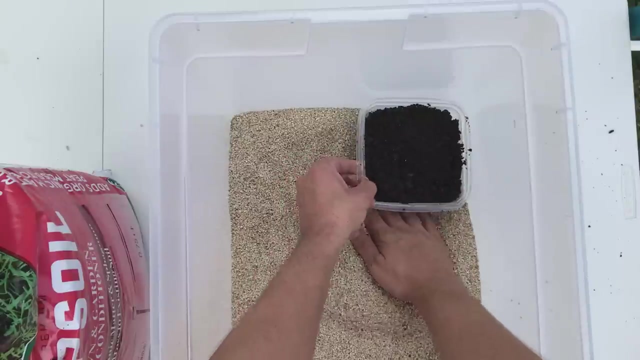 Just like that. Okay, now that's, that's where your crickets are going to lay their eggs. So let's take this, Find a corner, Kind of kind of burry a little bit, Just kind of move, maneuver the bedding around there. 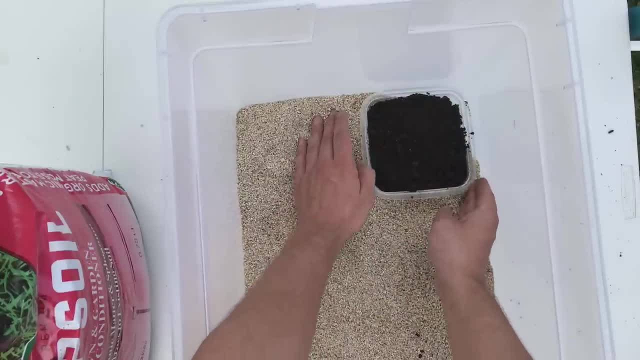 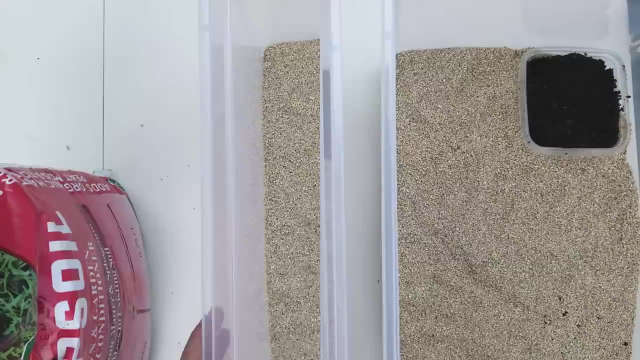 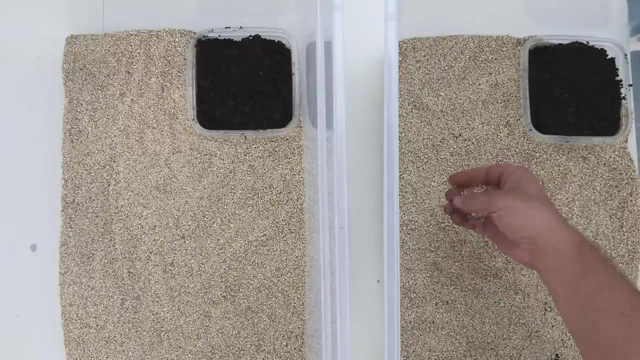 Kind of want to fill in the gaps. You don't want your crickets getting stuck back there. So there, Okay, here we have our two cricket habitats. Both of them, We have the same amount of the vermiculite for the bedding And we have our topsoil in the egg depository, where the 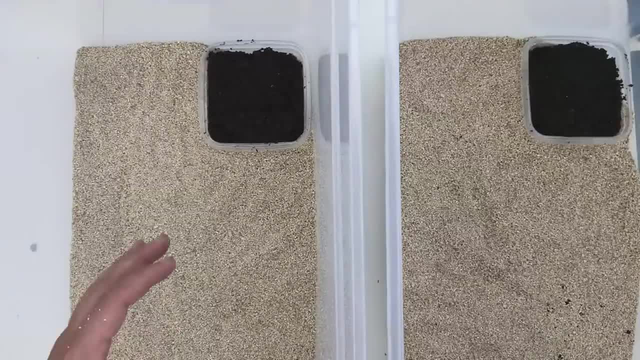 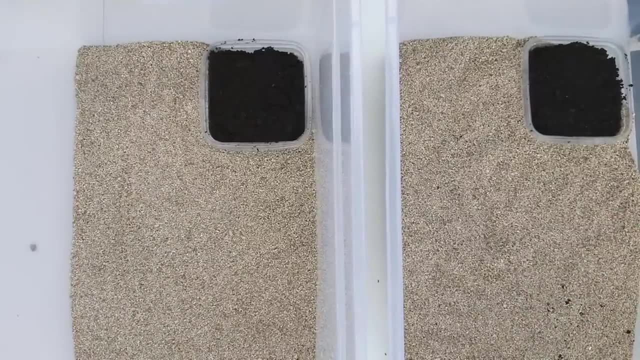 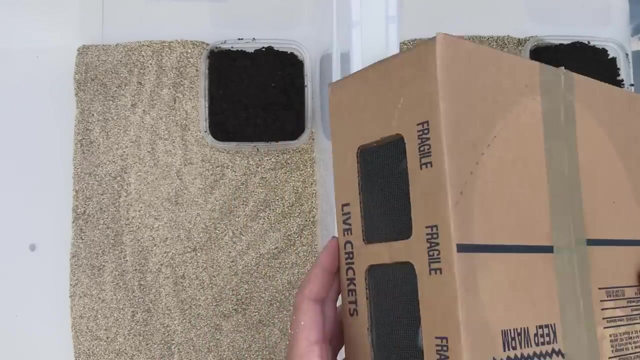 cricket- female crickets- will lay their eggs, So now it's time to introduce our crickets to their environment. Okay, so I'm going to pretend to be you guys. I just got a thousand crickets in the mail, So, as you can see, we package them in screen containers. And I got: Oh, that's a good. thousand quarter inch crickets. quarter inch crickets. they're only about seven days old. they're not quite ready to breed yet. if you're looking for crickets to breed right away, then you might want to consider, like the 5- 8 inch, that they're about 10 to 12 days old. the reason I recommend going with something: 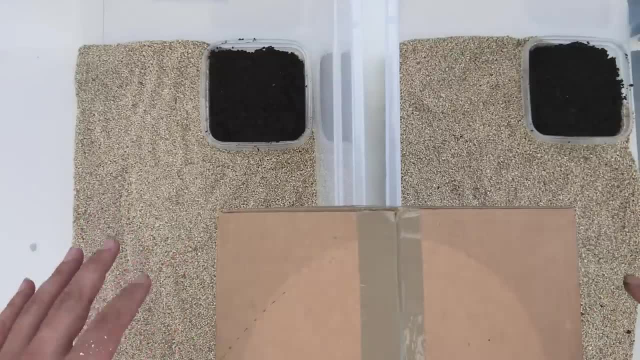 a little younger, because then it gives them time to acclimate to their new environment. after the transit can get a little stressed out and if they're sexually active they might not adjust as quickly as younger crickets can. so that's why I think the quarter inch- starting with quarter inch- might be a better plan than going right away with crickets that can start breeding right away. so here I already open up the box. we already got some Lucy's: one egg crate put it in there with the other egg crate, put it in the other one and just gonna pop them in. you know the transits rough on them, so they're gonna. 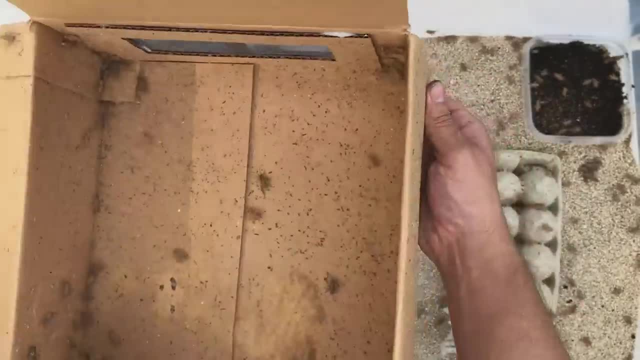 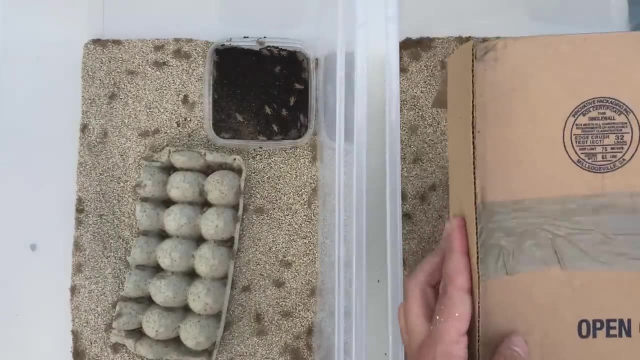 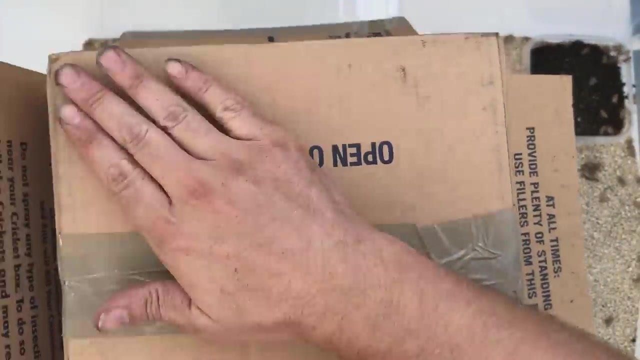 be jumping, not sure what's going on. so they're gonna be jumping everywhere and, and, and, and, and. you know if you're capable of getting every last cricket? and tell me your secrets, because I'm not sure how to exactly. you know how to not get some. 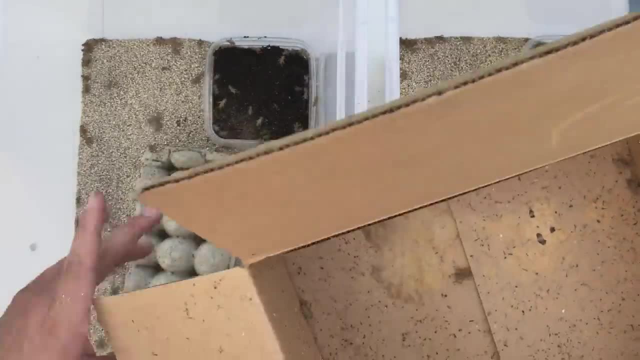 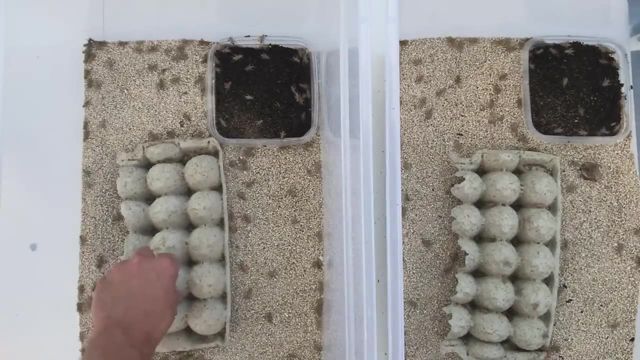 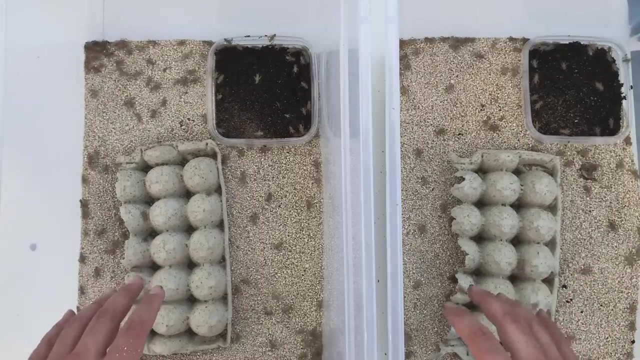 runaway crickets. okay, so that was a box of a thousand and you know, I don't know exactly if I exactly have 500 apiece, but it's good enough. so, after the transit, these crickets are severely damaged and they're not going to be able to breed. 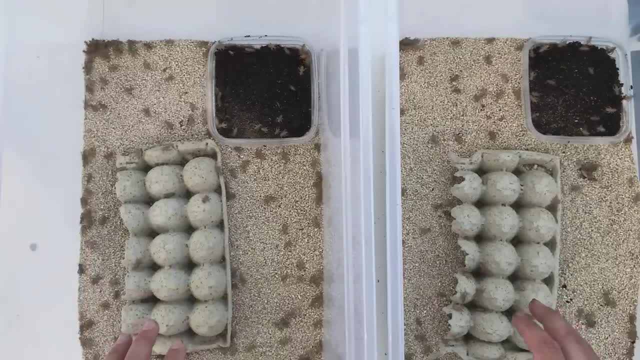 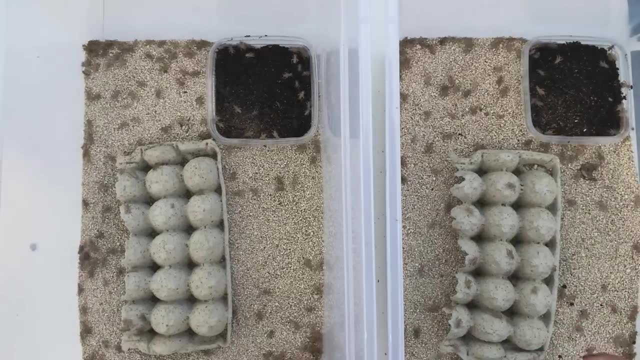 these crickets are severely damaged and they're not going to be able to breed. these crickets are severely damaged and they're not going to be able to breed Hillary, more than any other water titan finger, their more than any other water titan finger. You'll need to use the right nutrients is best to take care of your crickets. 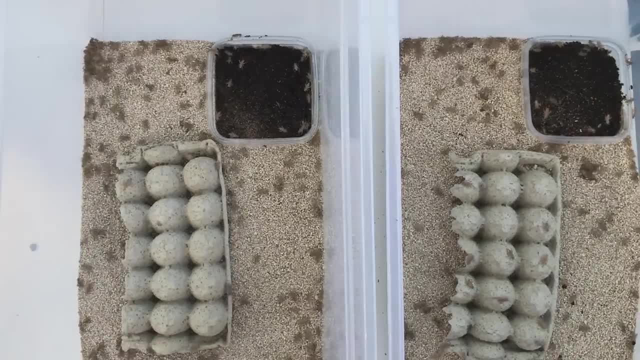 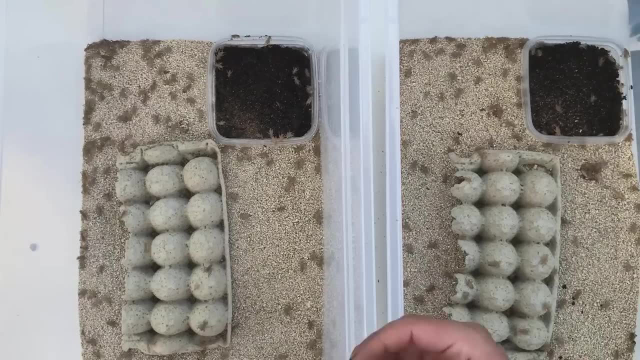 listen to what I say and if you want to try different plants and water, they're a whole, possibly different business. so be patient and you know there's that love for your hope andsuction. so we just end up taking a half a responds, but no problem, and sure enough, this video is gonna continue. we'll be learning more. 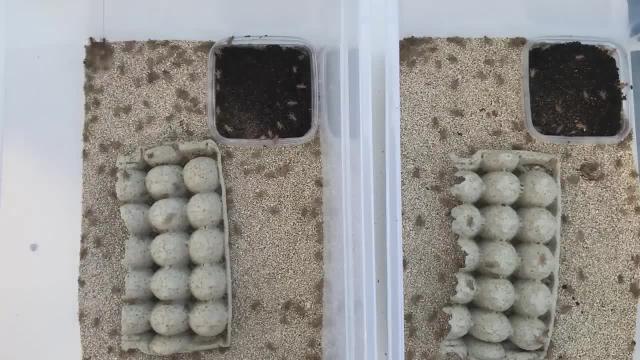 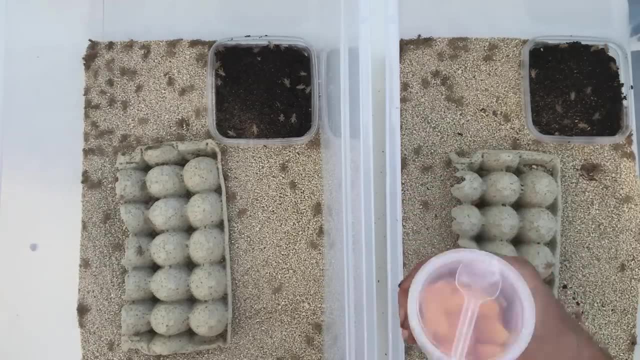 as we keep on exploring the weeds that the wild grass seemed to do with them after the long transit. and you know, something I actually like are these little cups, these little cups of oranges. I see they sell these for a dollar at the dollar store. so you know, these cups, they're saturated in water. I already 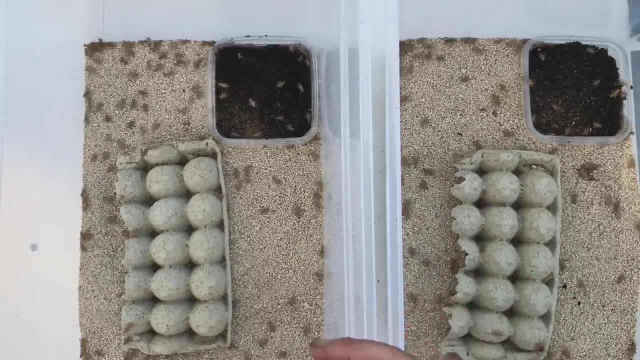 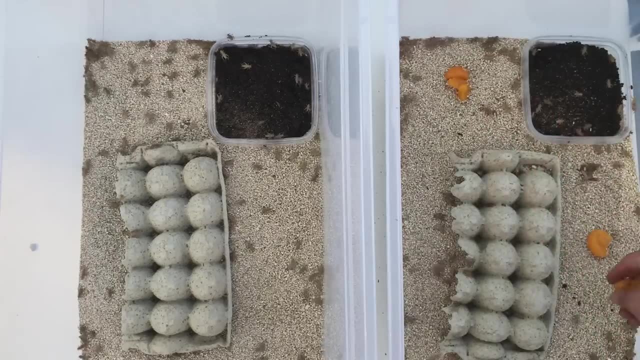 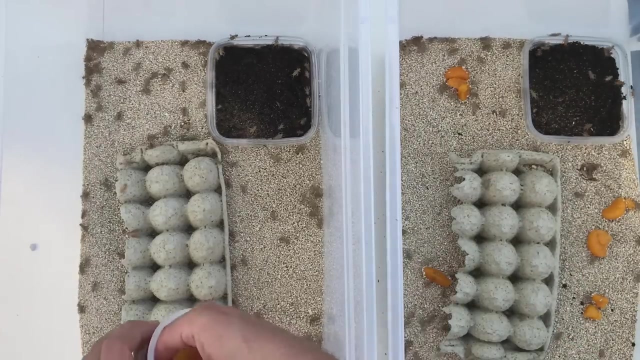 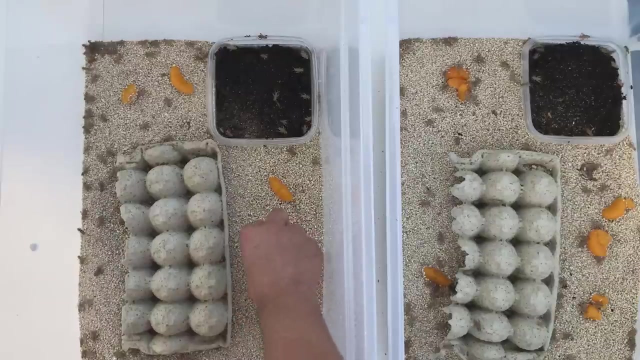 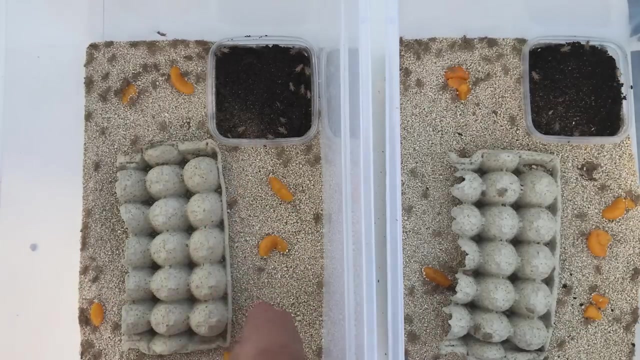 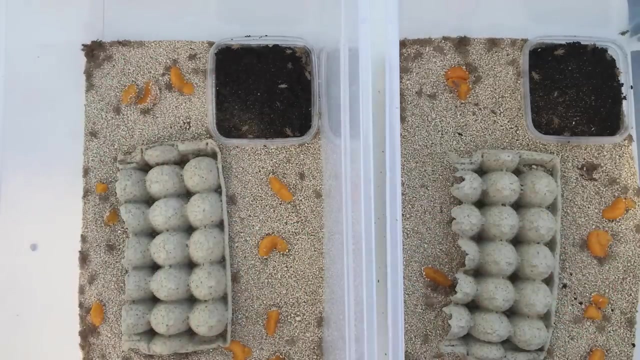 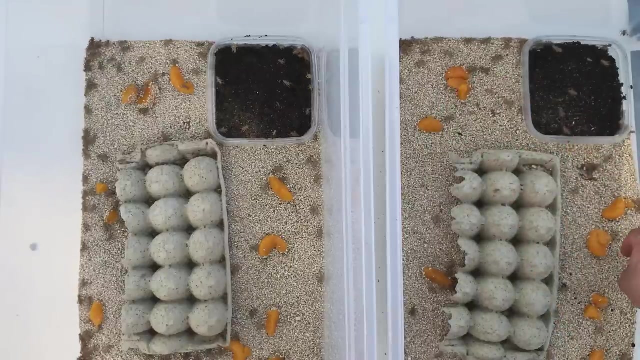 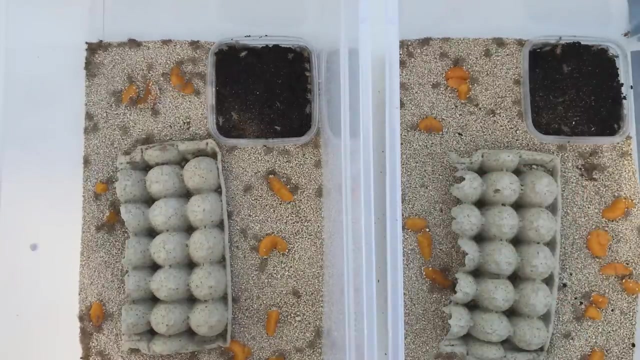 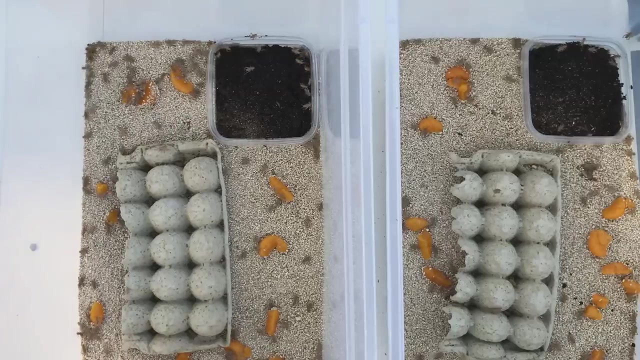 dumped out the juice, so I'm just gonna go ahead and put these mandarins inside the cricket habitat and in a few minutes, you're gonna see these crickets swarming around these mandarins because they are thirsty. okay, so, as you can see, our crickets are fed. they are starting to swarm the. 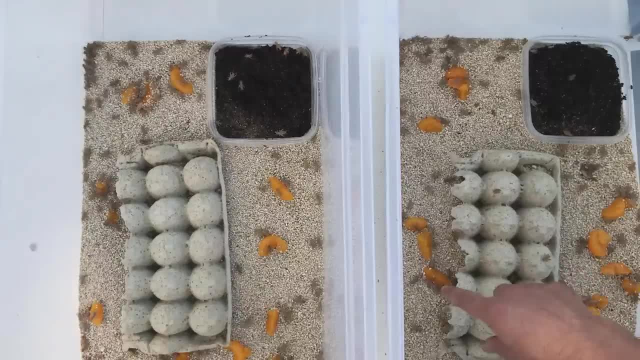 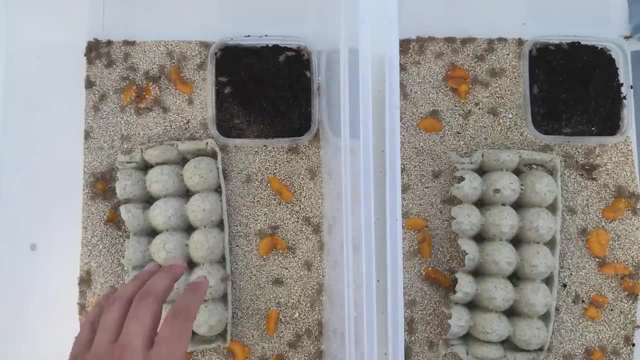 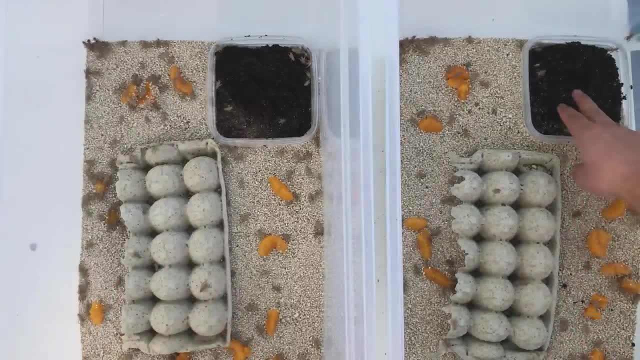 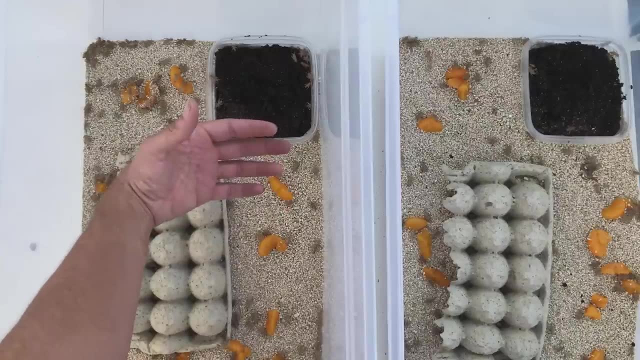 estásense in nutrition and so really, what they're gonna live in here for about a week. so in one week I'm gonna come back and I'm gonna check in on their tubs of topsoil. what I'm gonna be looking forиход eggs and as I start to, 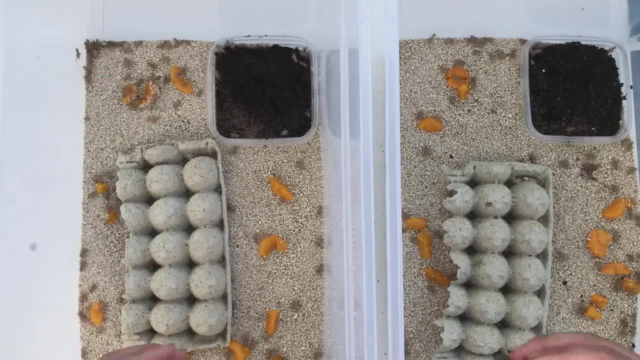 see more and more cricket eggs. there's a point where they're no longer in the late cricket eggs in this cuz it's gonna be too many. so what I'm what I will, then any other crickets. then those crickets will hatch and you'll have your pinhead. 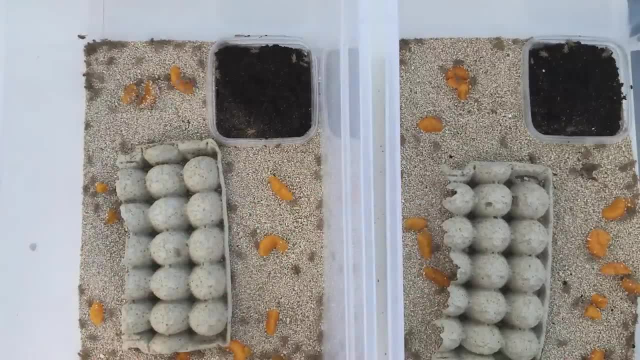 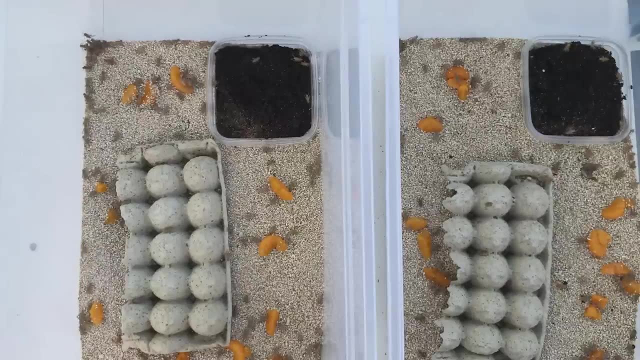 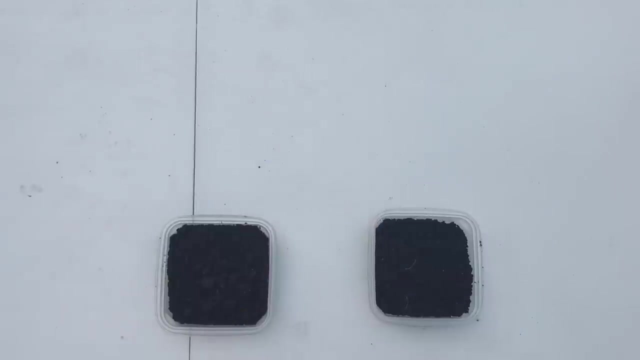 crickets isolated all by themselves, and so you know, about a week after that happens, I'll film it, let you guys see it and we'll review it. so talk to you then. okay guys, we're back. it has been about two weeks since we put together our 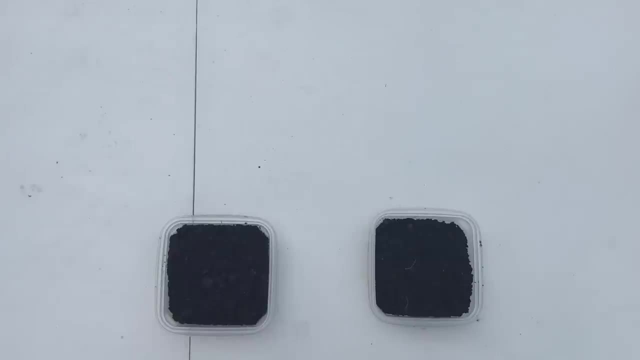 rearing bins and that has allowed our crickets about seven to ten days to breed and lay eggs inside their egg containers. so what we have here: we took out the two containers and now it's time to make the incubator. so the incubator bin is very similar to the rearing bin, but it's probably a little simpler to. 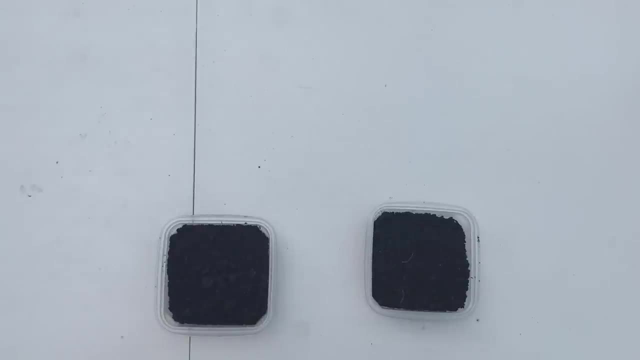 make. it requires less, less actual material. now, one thing I wanted to go over that I didn't mention before. I wanted to go over that I didn't mention before was, as your egg bins have been sitting inside the rearing bins, it's a good idea just to check on their moisture now. you don't need a hydrometer or anything. 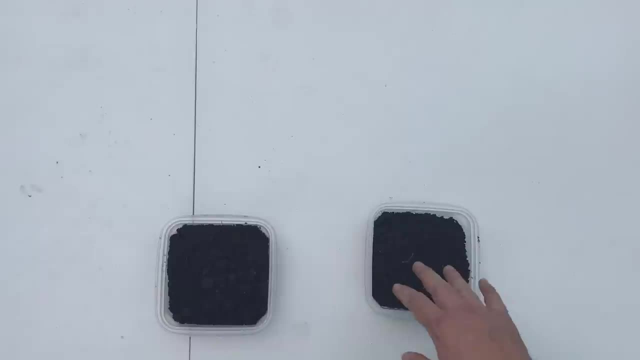 sophisticated. you can just use your hands and see if it's damp, just make sure it has a nice dark color to it and if not, all you need to do is just take a spray bottle filled with water and just just want to spray down. spray the topsoil down. that'll help keep the keep the topsoil nice and damp. 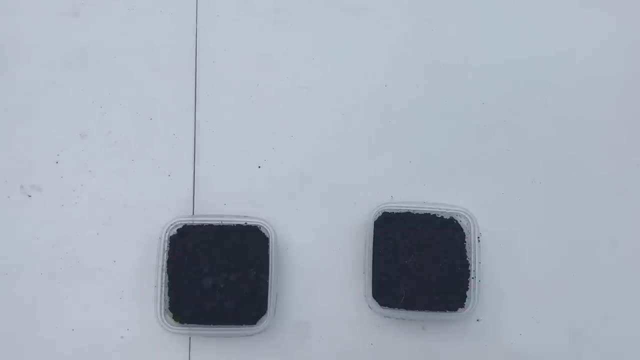 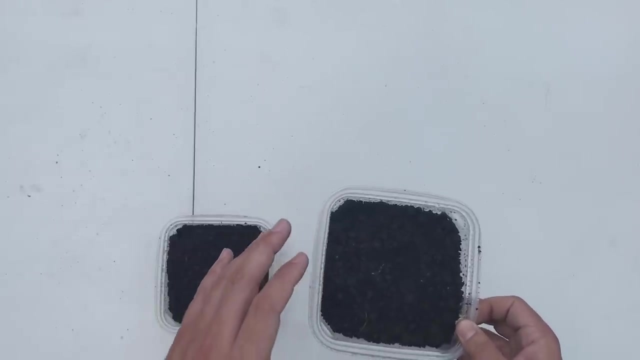 and it'll greatly increase the chances of all the eggs hatching successfully, which will increase your cricket yield. so you know. so now that we've removed our egg containers from the rearing bins, these containers are sat, are filled with eggs. now you're not gonna see any on the top. the crickets like to burrow into the. 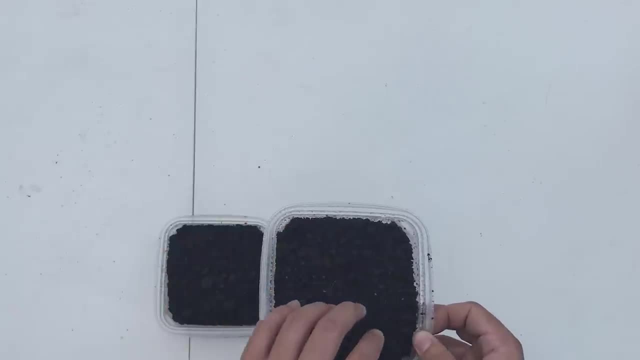 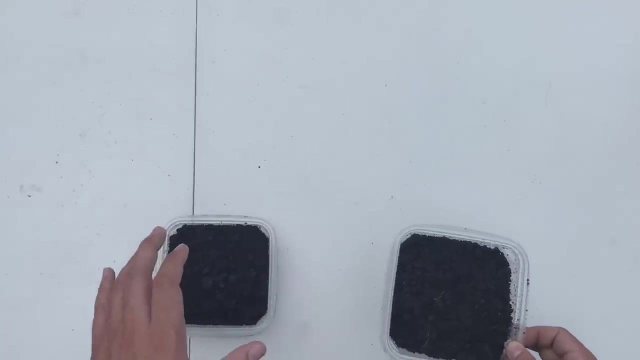 topsoil and lay their eggs down into the topsoil. so just just give it about seven weeks- I'm sorry, seven days after your 3, 8 inch crickets have been resting inside their breeding, the rearing bin, and you'll know that it's time to get their 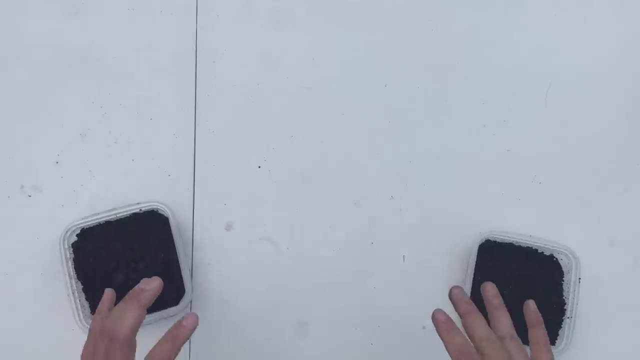 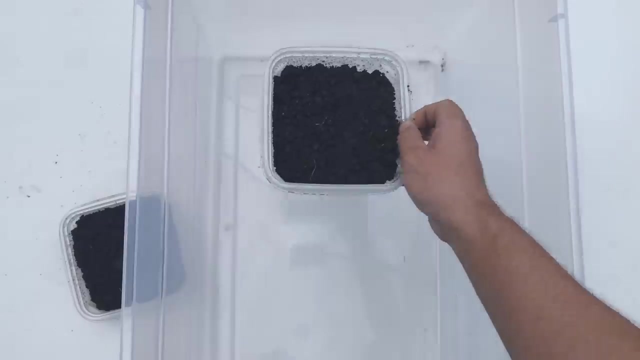 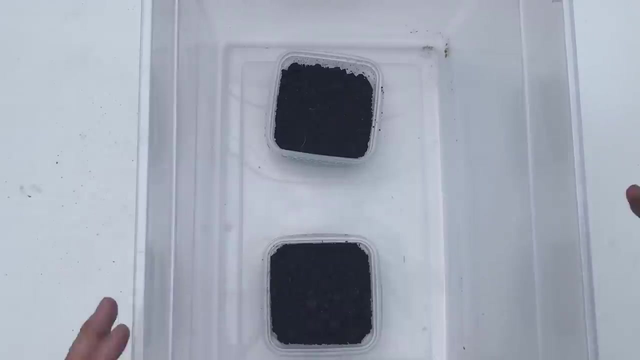 incubator bin put together and putting their incubator bin is. it's a lot simpler than the rearing bin. so all you need to do is take another container just like you, similar to the rearing bin, and just place in the egg crate and that's all you do. a container like this you could actually 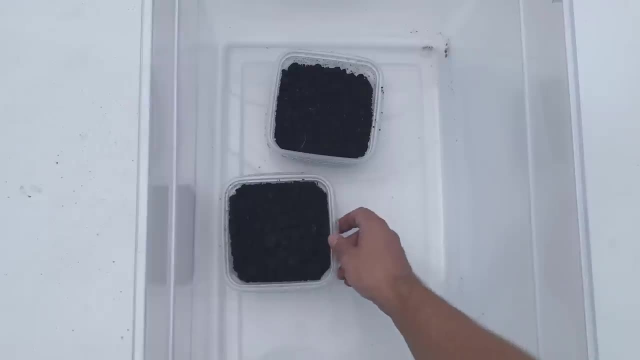 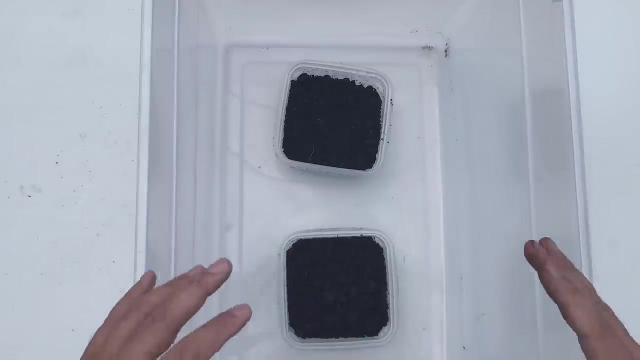 fit. there's enough space in here to fit two more, but since we only made two, we're just gonna put two in here for our demonstration. now you can definitely just keep it like this, but what you're gonna want to do is just take another container like this and put that in the rearing bin. now you're gonna want to. 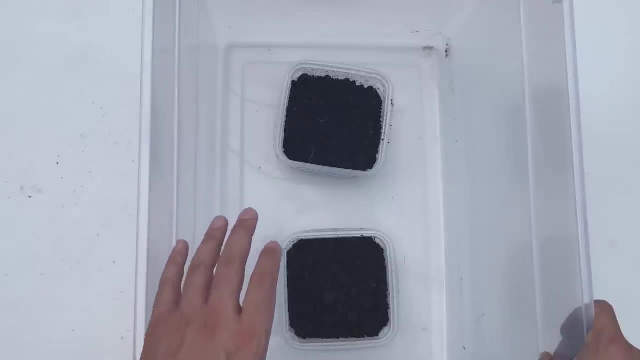 put the container back in again, so you'll want to put that inside the rearing bin. there we go now. you'll want to put that back in there so you can just put your rearing bin on top of the container and its gonna help you with that. 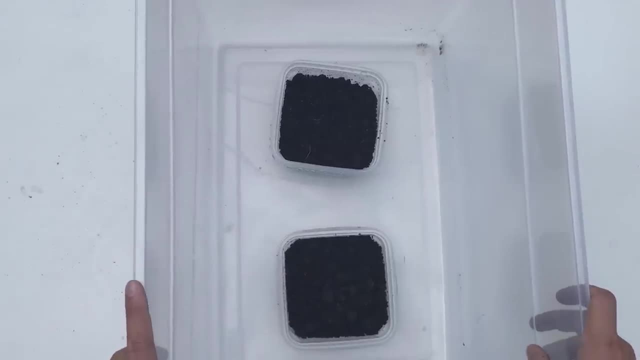 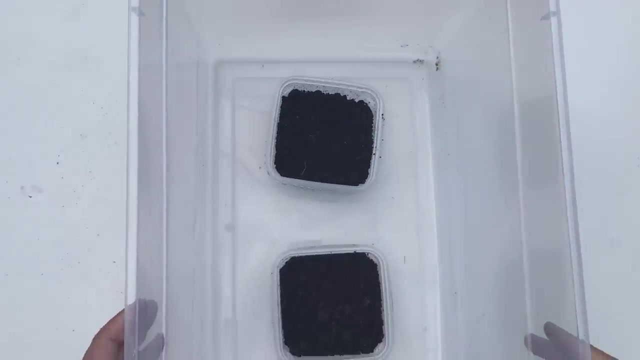 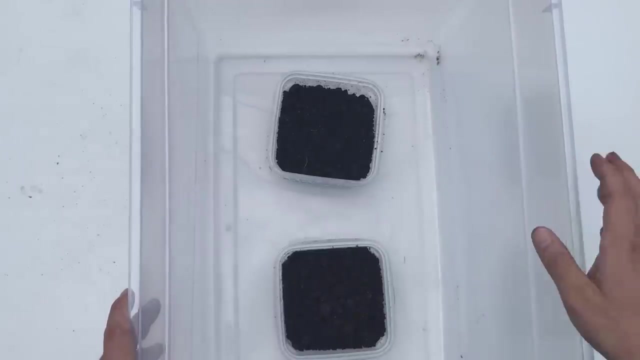 rearing it up. now the next step that you're gonna wanna do is locate this into someplace that that has a consistent temperature of about 90 degrees. these incubators, these eggs, are gonna need 90 degree temperatures For your pets and place it on top. The only issue with that is there's- you're gonna be. 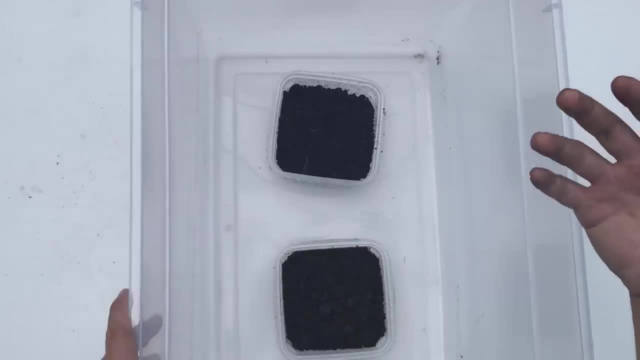 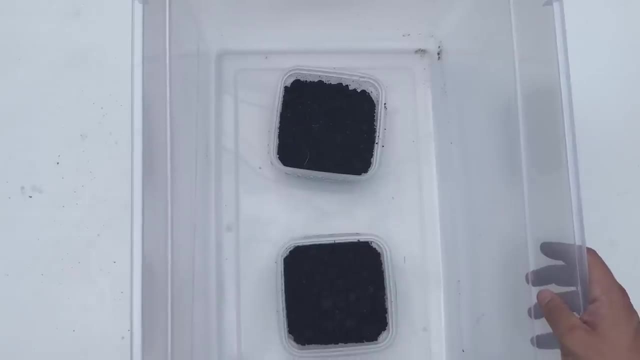 Dehydrating your topsoil faster than you would if you didn't need it. So just make sure you always have a water bottle. You're checking it every one, Every one day or two days, and just make sure that it looks damp on the surface. 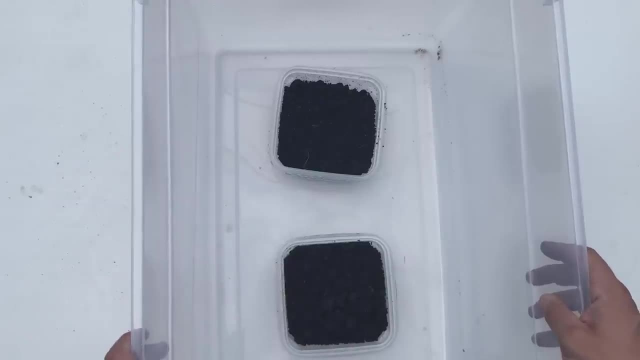 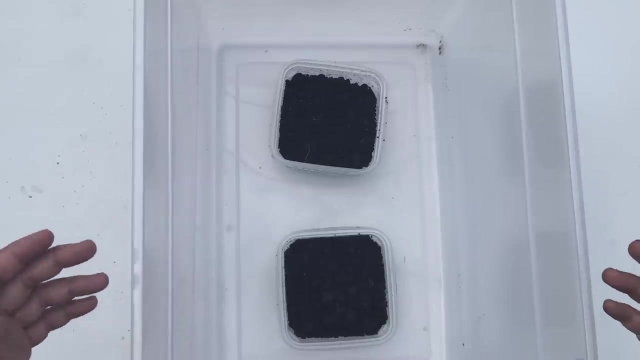 You don't want to fish your hands through it too much because you could disturb the eggs. But um, you know, once you have that set, Just let this sit for about a week and after a week you'll start seeing some crickets slowly start to hatch out and 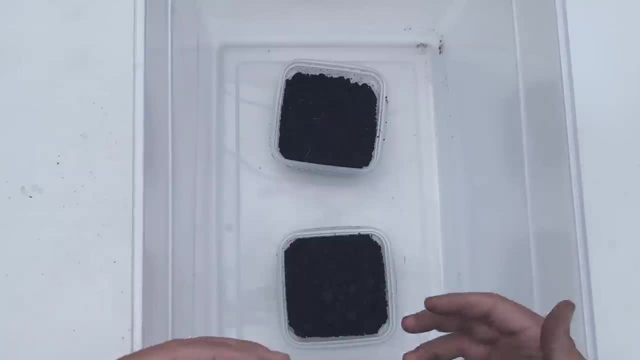 You know it'll take. you'll probably start hatching about a hundred a day and soon enough This whole thing will be filled with little pinhead crickets And once you have your pinhead crickets, you just remove them into a new rear-end container, like we made two weeks ago, and 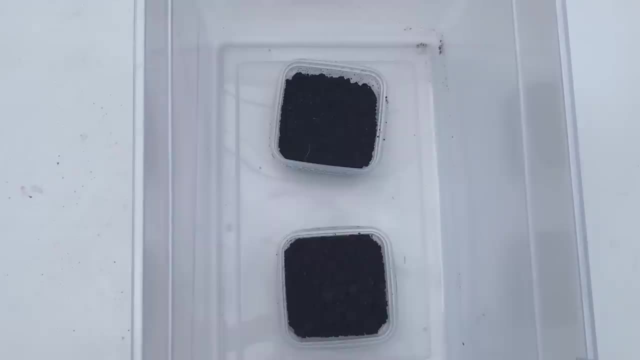 Just allow them to grow, allow them to propagate and just make sure you're feeding them the same Way, and that's how you start your cycle. That's how you start your cricket breeding cycle. So that's: we're just gonna give this bin seven days and see what happens. 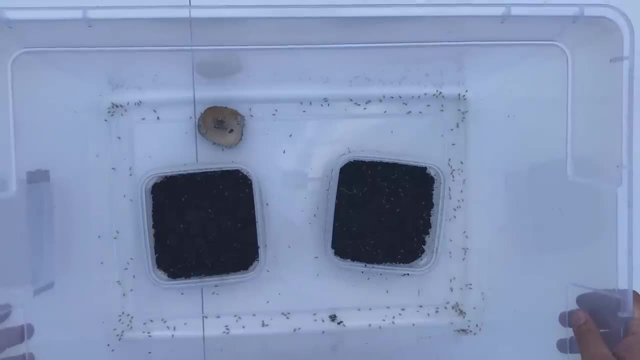 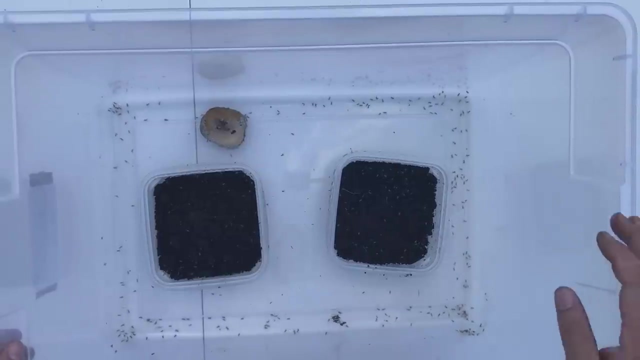 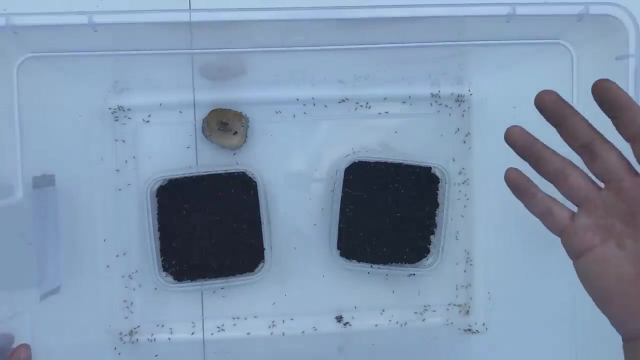 Okay, guys, welcome back. and so here's our incubator bin. We have had it sitting for about eight days so far and, as you can see, we are seeing some pinhead crickets start to start to hatch from their eggs and start to Habitate inside the. 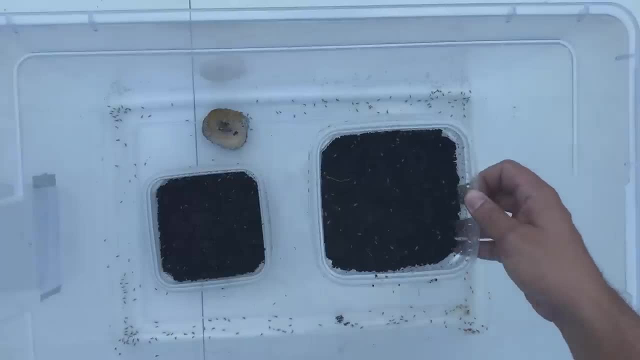 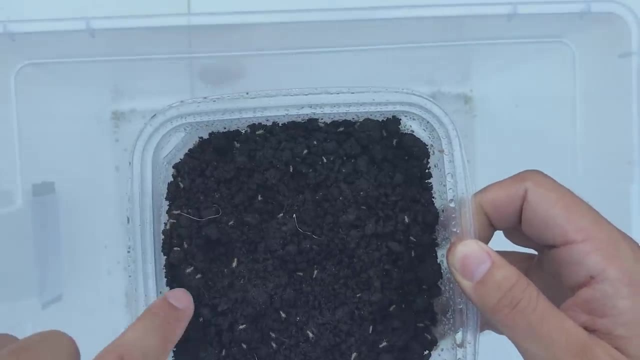 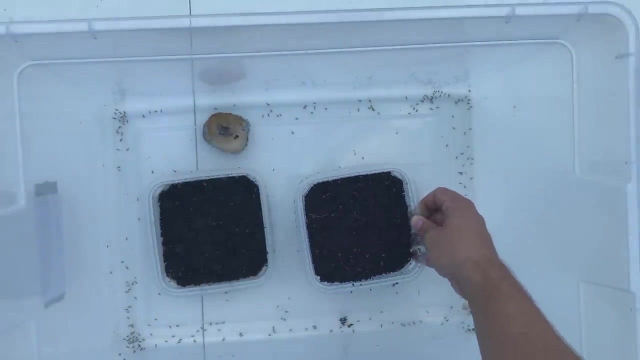 Our incubator. here's a close-up. You can see them hopping around a little bit, So Just always got to make sure your soil is moist, because there's still eggs to hatch inside of there. I'm probably gonna squish a few when I put this back down. 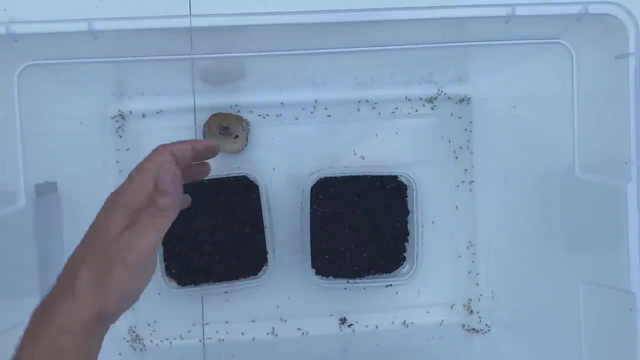 You know what you can do. you can give potato slices That will help them, that can feed them, Or you can go with some orange slices, Or even consider watermelon Juicier the better. but we just had some some rotten potato sitting around, So I just kind of use that up. 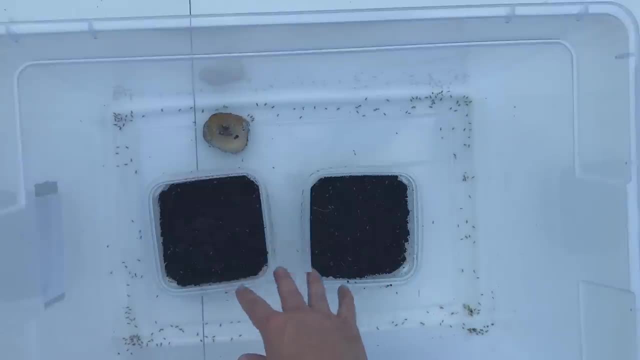 And same thing. just want to make sure you're lightly misting this now. this, this still looks fine, So I'm not gonna mist it, but Your crickets also need water. So Tub like this: There's a little, there's a little channel around the perimeter. 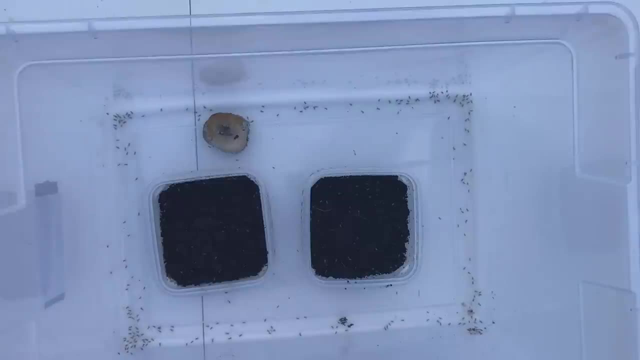 Some might go ahead actually and just missed it a little bit. Some might go ahead actually and just missed it a little bit. what I expect to happen will be: the water will run down in the channel and Our little crickets can Just get their hydration and, as you can see, they're starting to go towards the water already.